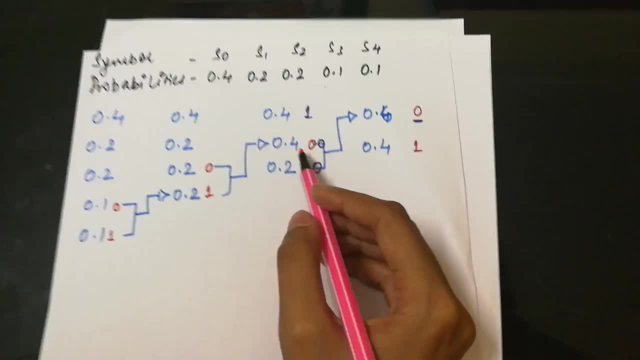 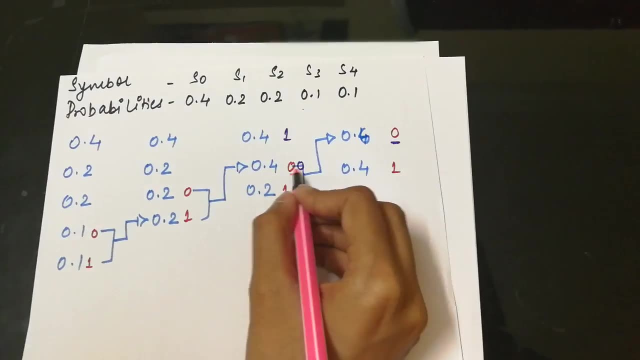 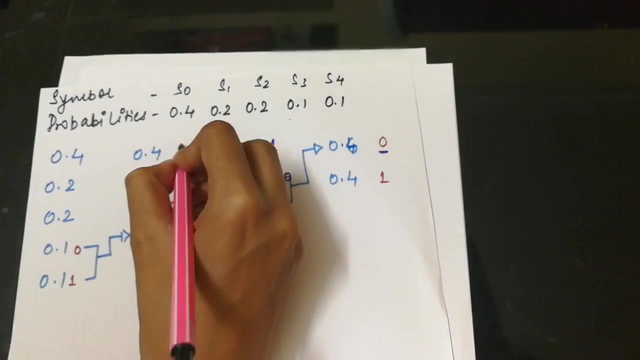 in front of 0.4.. Now 0.4 is the result of 0.2 and 0.2.. In front of 0.4 we have these two, So these two would be written down here And this 1,0 is here Now. this 0.2 is the. 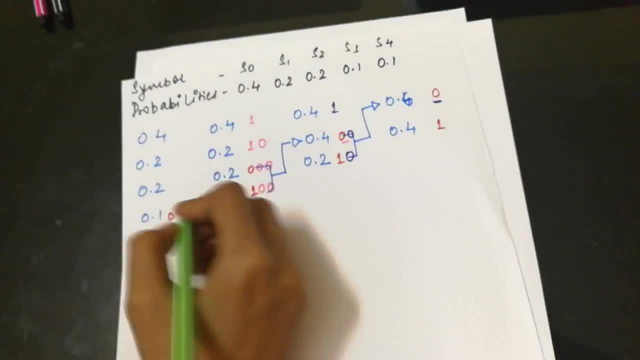 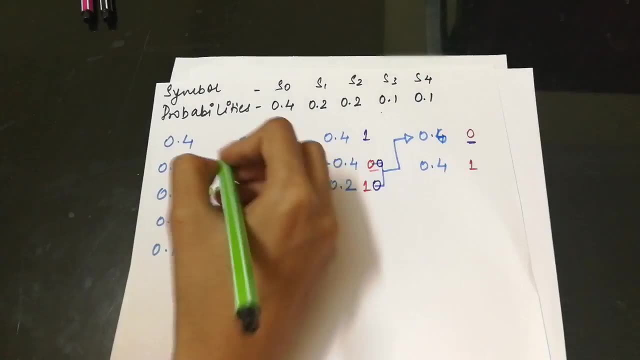 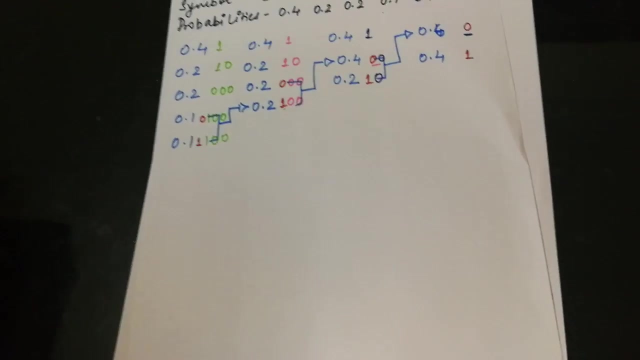 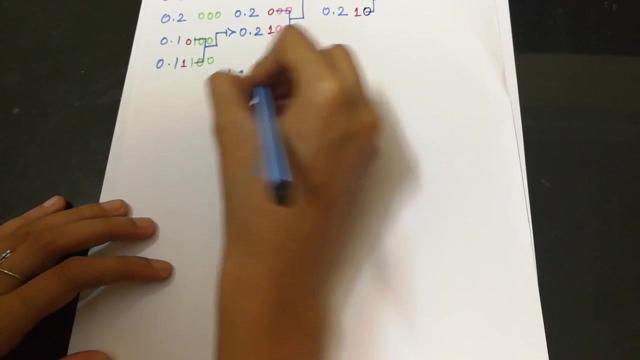 result of these two probabilities, Here we have 1,0,0.. So we write 1,0,0 and this are written here. Now, this is the first step that we have done. Now we start by calculating the length. The length is given as the summation of i is equal. 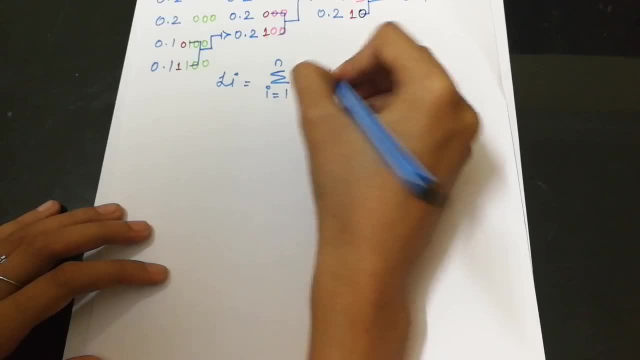 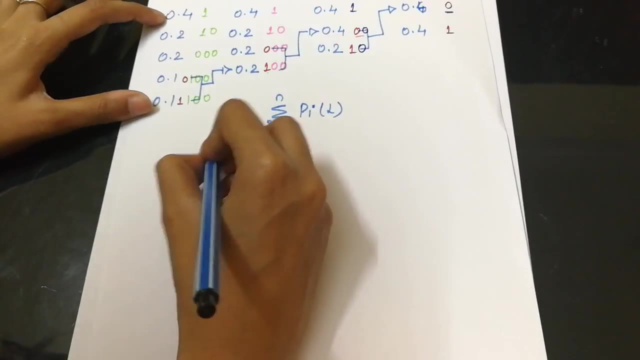 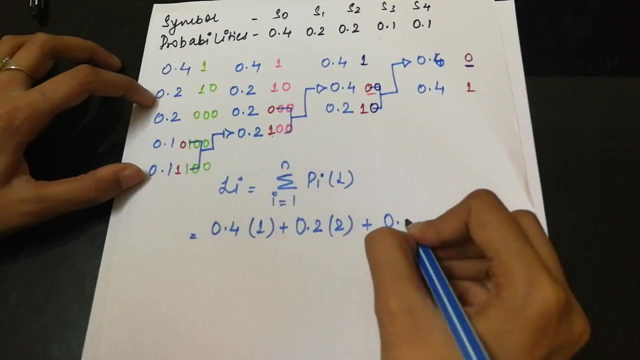 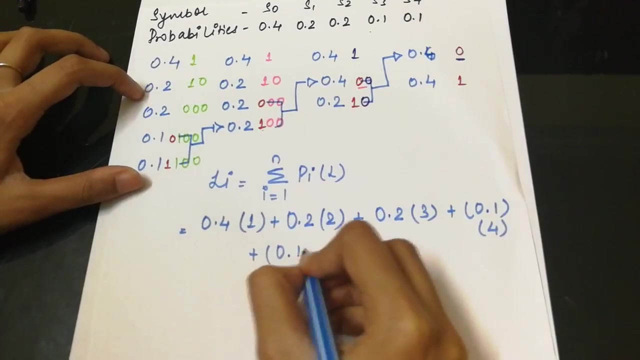 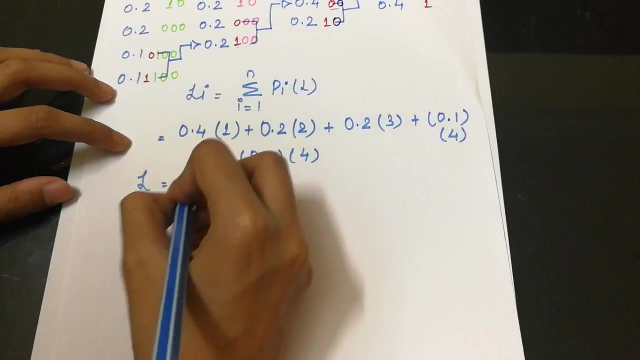 to 1 to n probabilities into the length. This l is the code length of the probabilities. This would become 0.4 into the length 1,, 0.2 into the length, 0.4 into the length 3.. now, on adding this, we get L is equal to 2.2. now we start by entropy calculation entropy. 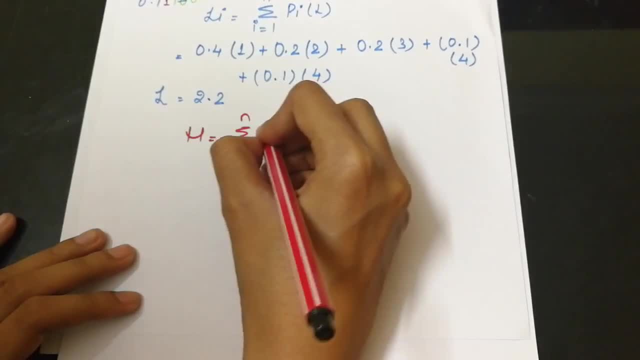 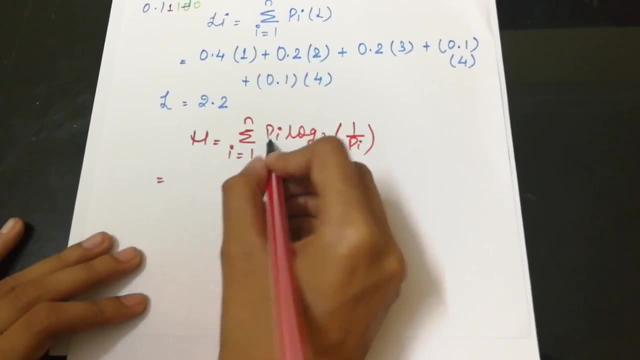 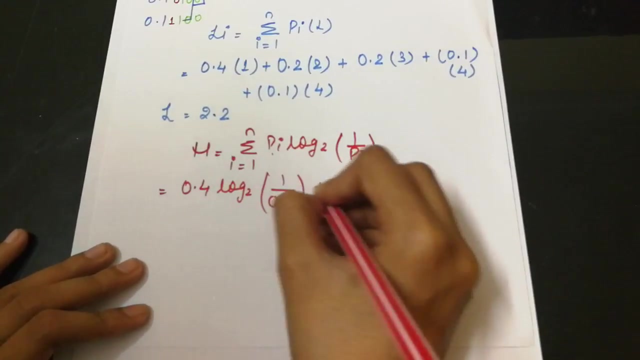 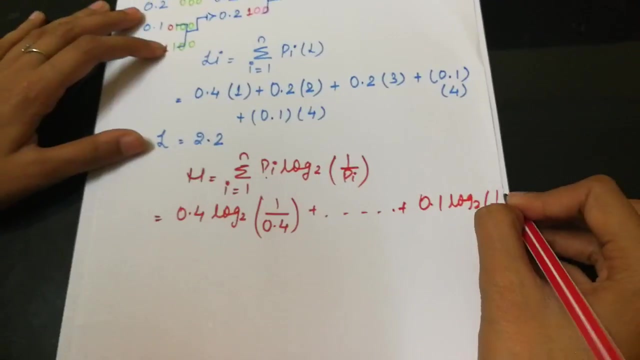 is given by summation of I is equal to 1 to N PI. log base of 2: 1 upon PI. this will give PI is your probabilities: 0.4 log base: 2: 1 upon 0.4. Tim 0.1 log base: 2: 0.1. now on this. 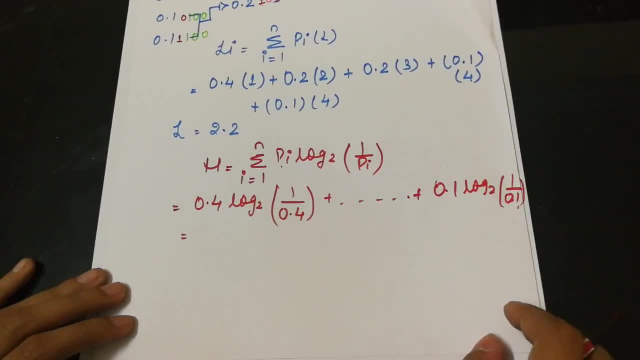 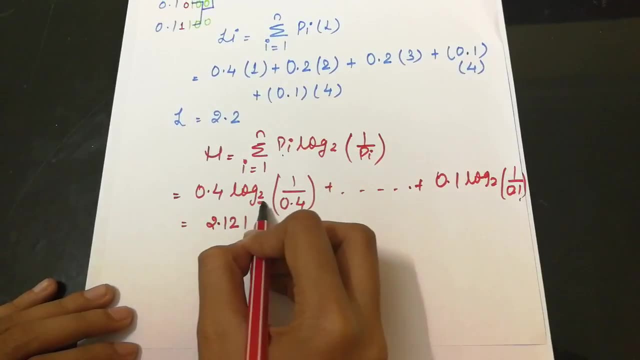 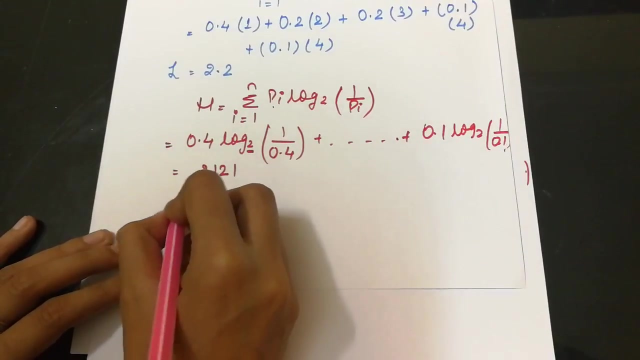 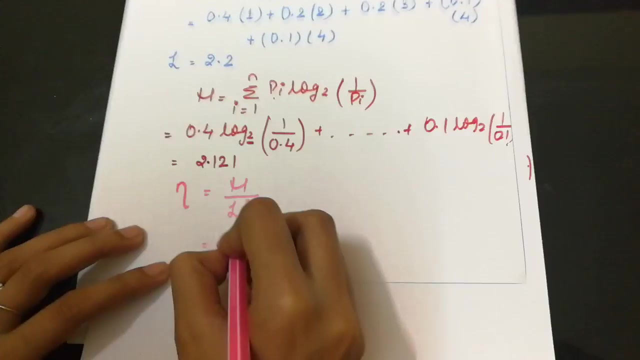 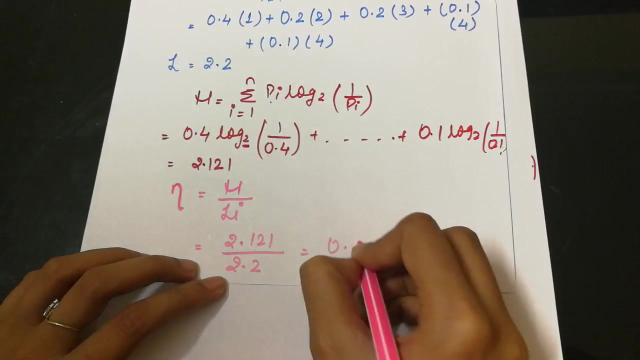 calculation: when you calculate this with your calculator, you get 2.121. it is very necessary to write log base 2 in your calculator. now, efficiency is given as eta. efficiency is denoted by aeta, which is given as entropy divided by depth, which is 2.121 divided by 2.2. on calculation of this, you get 0.96. now